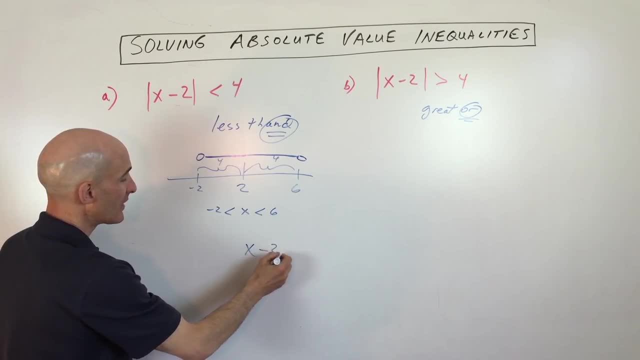 like this: if I had a less than inequality- okay, absolute value inequality- what I would do is I would write it as a compound inequality. I would say: whatever's in, the absolute value is less than four, and remember less than- and it's greater than the opposite of four. okay, so x minus two is in. 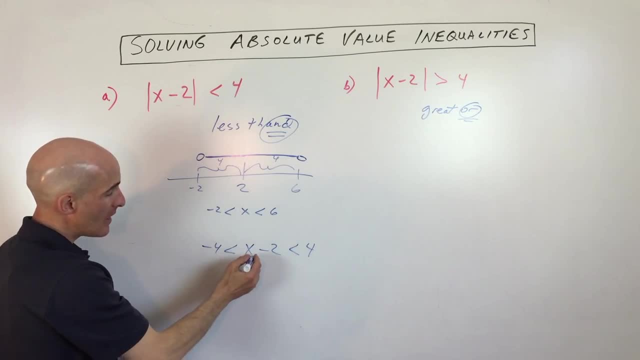 between those two, the negative and the positive value. then we're just trying to solve for x, we're trying to get it by itself. so we're going to add two to the right, the middle and the left, and if we do that we get negative. two is less than x is less than six. the same thing we got here by you. 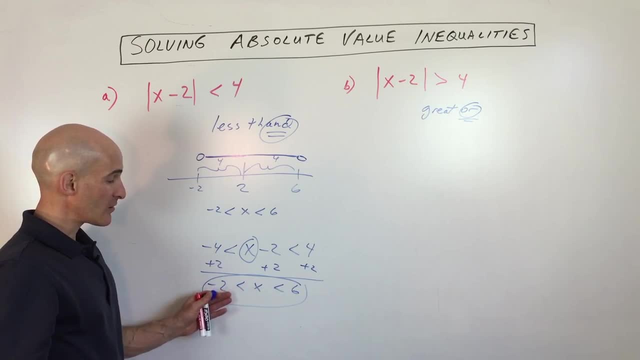 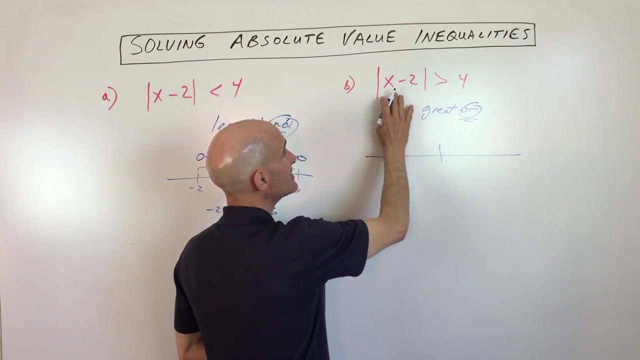 know, analyzing it geometrically. so x is greater than negative two and less than six. so remember less than and and you can write it as a compound inequality and just do it like we did this one. let's look at an or one now, same geometric interpretation. basically, we have the distance between some number and two. 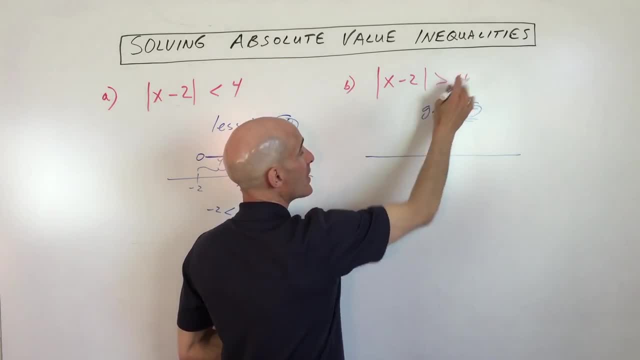 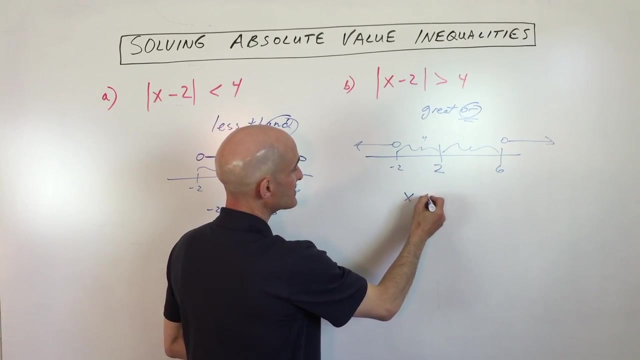 difference means the distance between some number and two is greater than four units away. so greater, of course, means further away, right? greater than four units away. okay, so you're gonna be like this, okay, so now, if we saw this on a number line, we would write: X is less than negative two or X is. 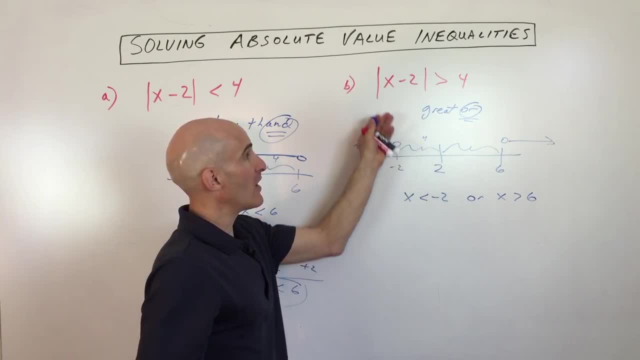 greater than six. great, or right now, you, like I said before, like you, might have a more complicated problem than this. it might not be so easy to graph it like I just did, so what you can do is you can use this algebra way of solving it. you're just going to split it up into two. 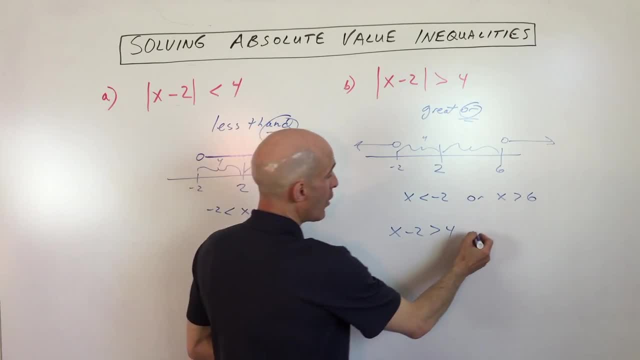 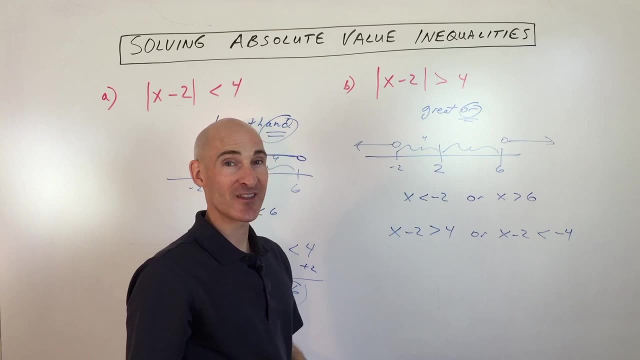 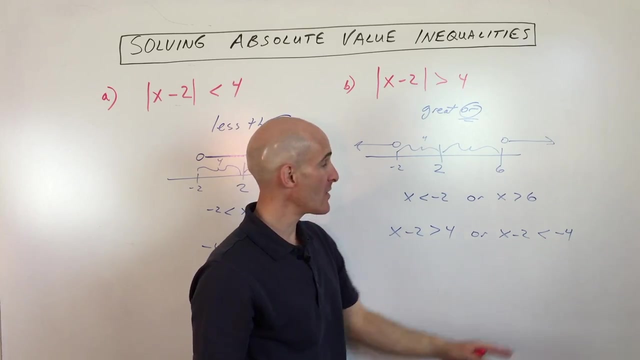 inequalities: x minus two is greater than four or x minus two is less than negative four. oh wait, a second. what did I do right there? I switch the inequality sign and I switch the sign of this number to the opposite. okay, now, this little. Now you might be wondering: okay, why did I do that? 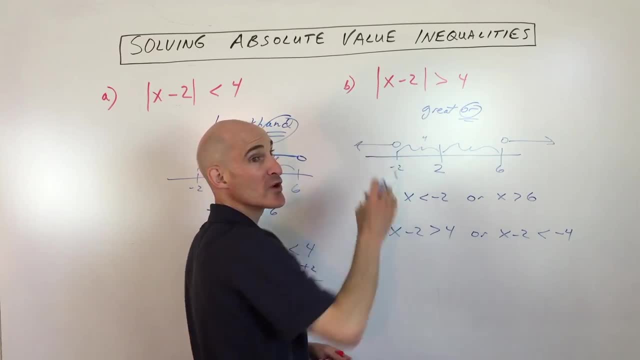 And let me see if I can explain Whatever is in the absolute value originally, before we took the absolute value right, making it positive. this could have been negative or it could have been positive. Now we're working backwards to find out what x was originally, before we took the absolute value.